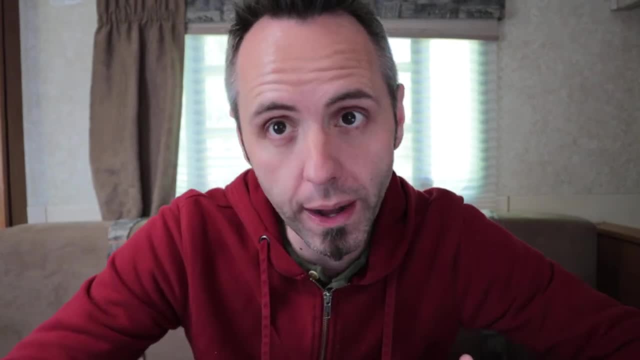 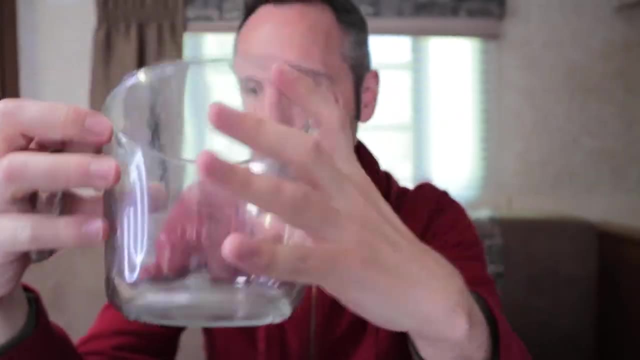 the dishwasher and have been through the microwave and all that type of stuff, and we noticed that the pyrex one was losing its stuff over um, over the anchor hawking one. so we were like, okay, should we try an anchor hawking one, because we need the big. 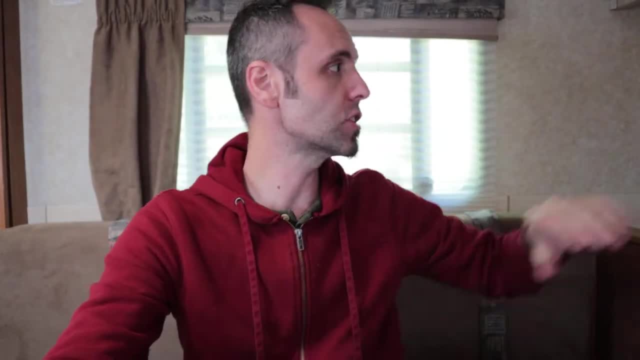 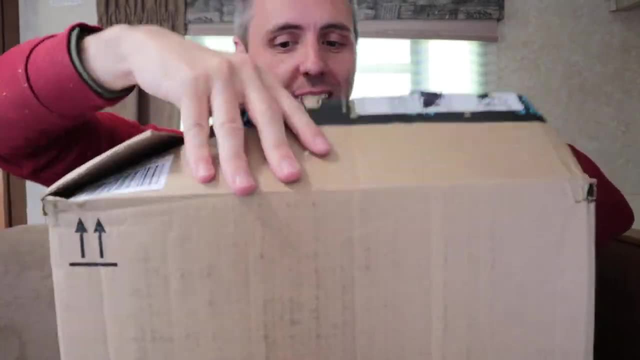 one. we need the bigger one, uh, for all the baking and stuff that we do, so in this box. right here we got our answer. let's see what we got here. first of all, hi, hide all the new dads out there. this is dad reviews. this is where i give you my unedited- hopefully more authentic look at the. 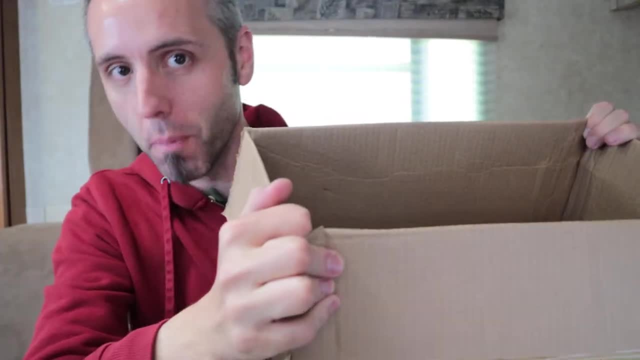 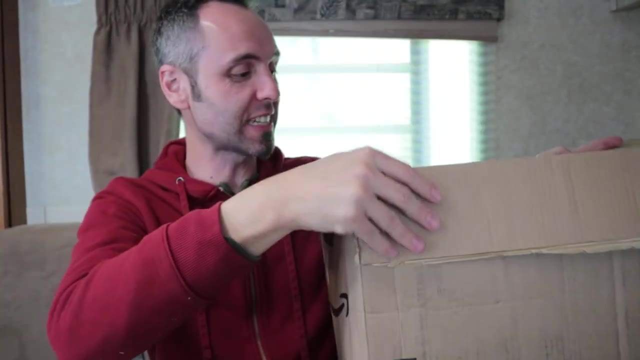 products that we like to use and have and hopefully don't lose markings over time so we can bake with. so if you're interested in that, you might want to consider clicking that subscribe button. watch this video all the way to the end so that you see everything about these measuring cups here. so we got this from amazon. i'll link it. 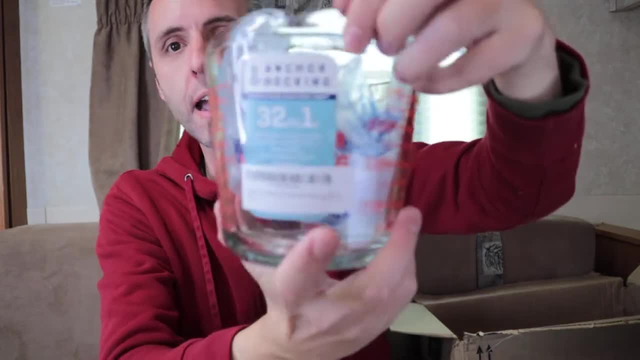 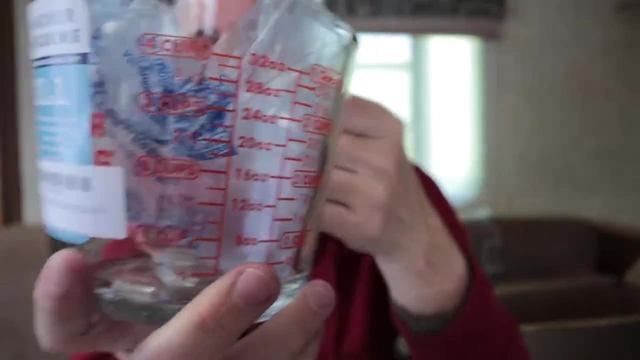 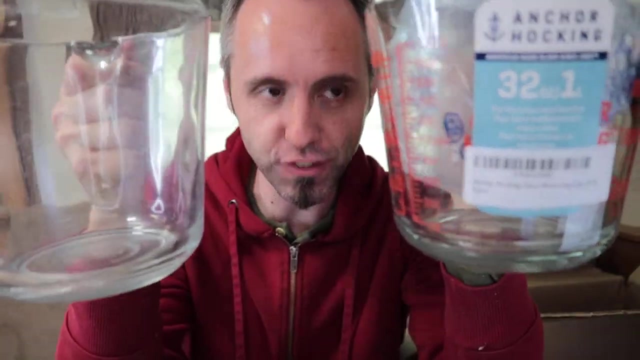 up down in the description below. but anchor hawking makes a 32 ounce four cup, one quart measuring cup here. that's glass and is extremely similar to this pyrex one here. so i wanted to kind of do a little versatile versus video here, because now i have apples to apples here. right, this was a little more apples. 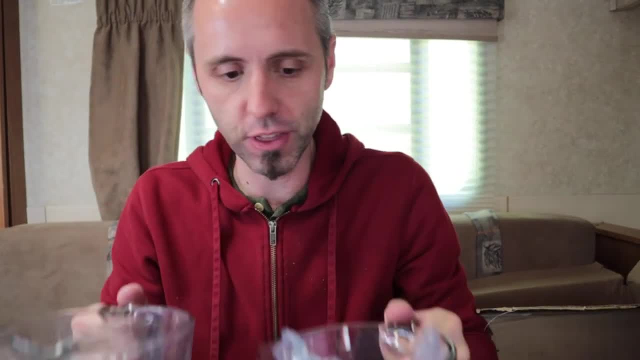 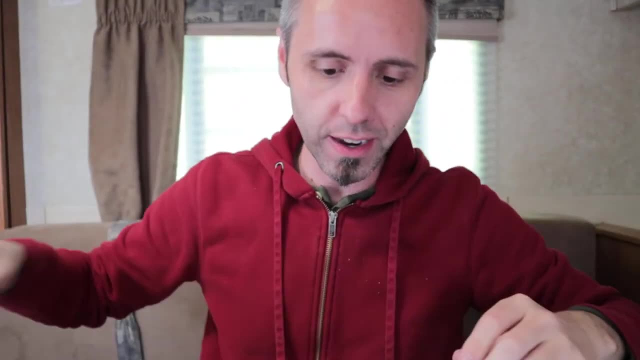 to orange, because this is a smaller one. but now i can really get a feel for everything that we have. let me get rid of this thing. now i can get a feel for everything that we have here. first of all, let's get rid of that. got that urn there. um, first thing that i noticed is that they- of course they have. 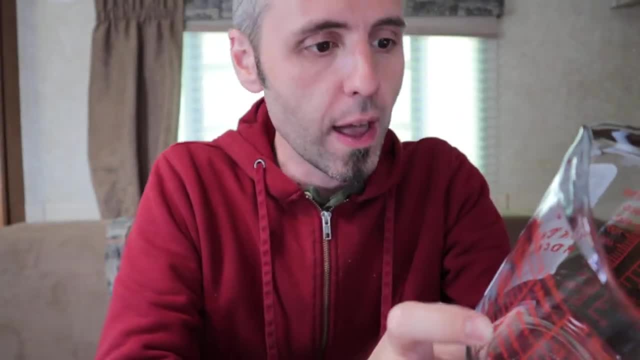 the label on their anchor hawking glass measuring cup: 32 ounces new uh one liter for microwave and oven use. it says it also in a few different languages. right there, do you guys know how to say this in any other language? i don't know how to say it in any other language. i don't know how to. 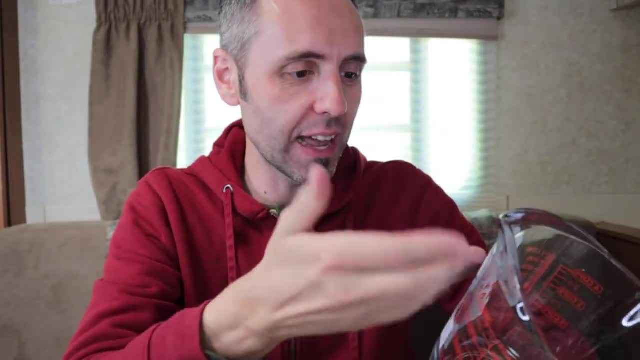 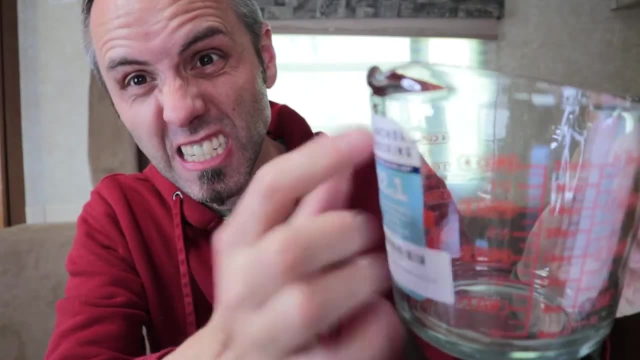 do um of any other languages, let me know down in the comments below. um, it's got the anchor hawking you can. this comes off, so let's see how easy the the peel is, and let's also see if it's going to leave any sticker residue on this thing. that's one thing that always frustrates me whenever. 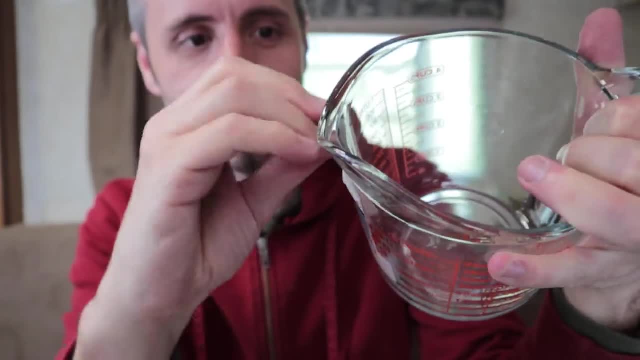 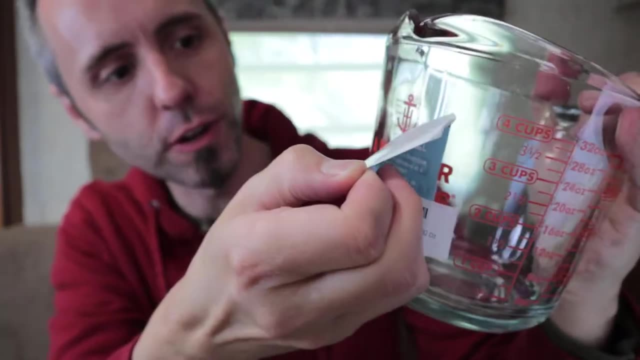 it comes to buying new uh dishes or glassware or anything like, that is the residue. you know, some stickers they have that easy to peel off type stuff, but uh, this one, oh yeah, this one's doing great. now i'm worried about that amazon sticker right there though. oh boy, let's see. oh, it says some. 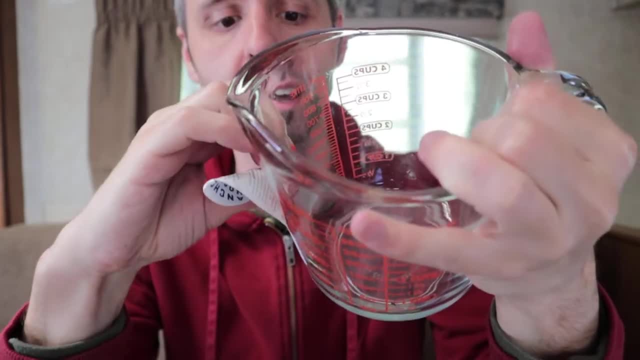 on the back here too, on the back of the stick. Oh no, come on, Amazon sticker, Come on, come on, Don't leave the residue. Okay, let me see if I'm just I'm using my nail right here to try and just peel it. 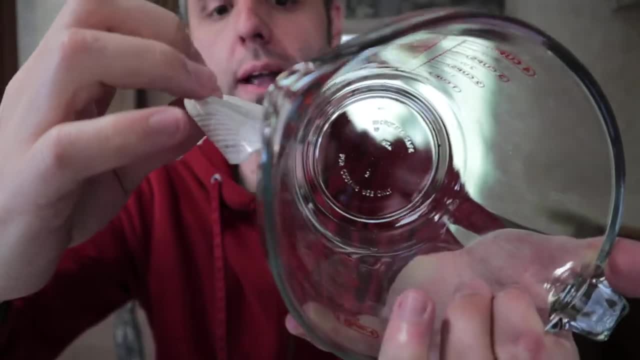 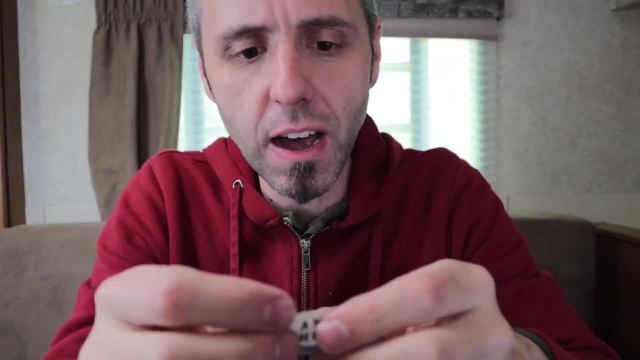 onto the Anchor Hawking sticker. It's not working. Okay, there we go, there we go. We got something. Oh oh, the Amazon sticker failed us again, Amazon, you failed us. So this says: for use in glass electric. 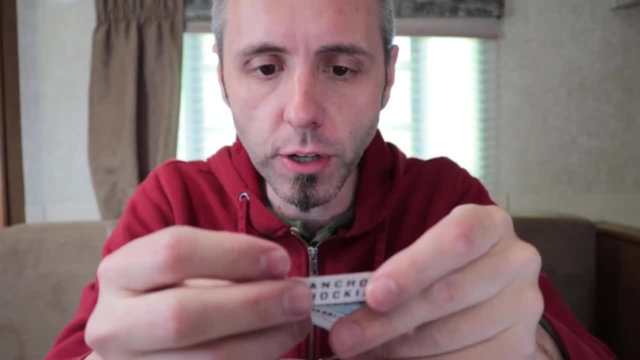 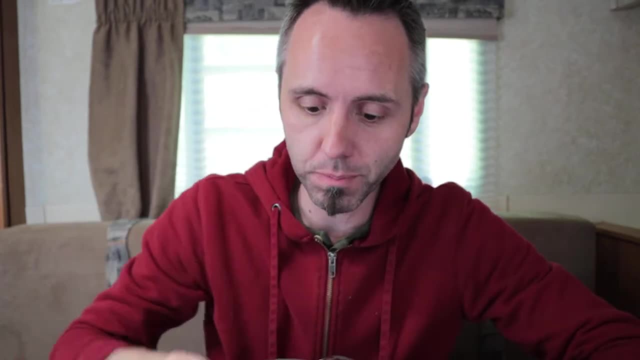 and microwave ovens. caution: do not use on top of stove or under a broiler. Breakage can occur. Actually, I was doing a little bit of research, keyword research- about this particular glass type stuff And there's keywords out there about the glass exploding. 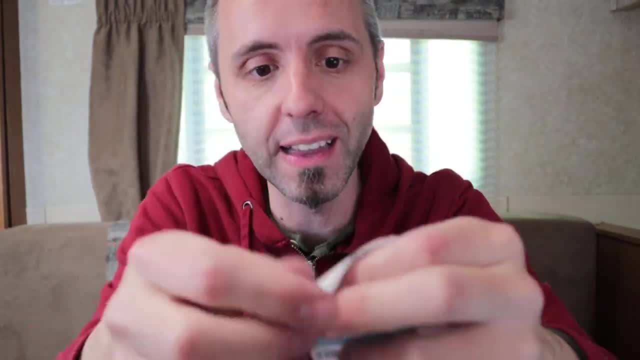 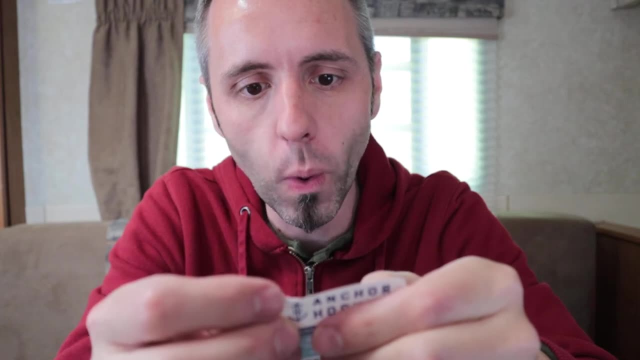 So that could be something that might happen if you put it in, like your oven or whatever. Do not add liquid to hot cup. Place a hot cup on a wet or cold surface or handle with a wet cloth. Avoid impact. handle with care. discontinue if chipped. 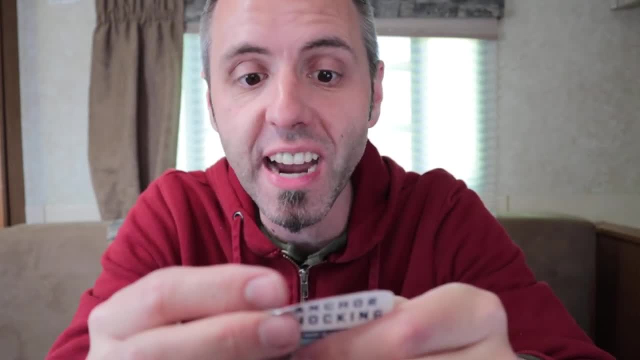 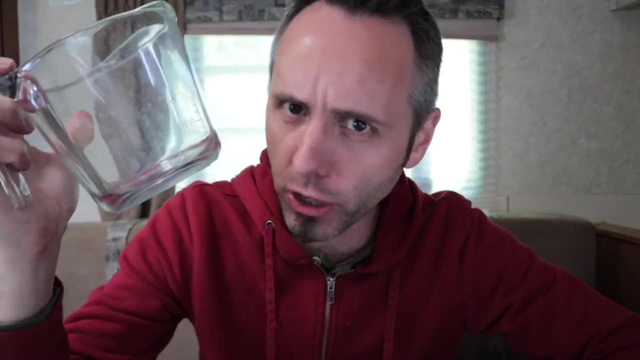 cracked or noticeably scratched Dishwasher safe. some detergents may remove the decoration and results in etching of the glass. Oh, that's very I wonder if that's what happened here. So I'd be curious to know what kind of dishwasher detergent. 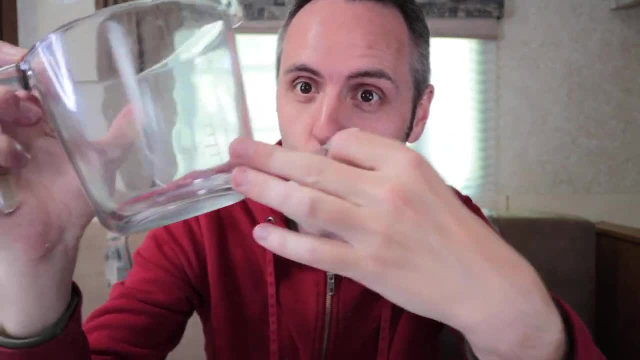 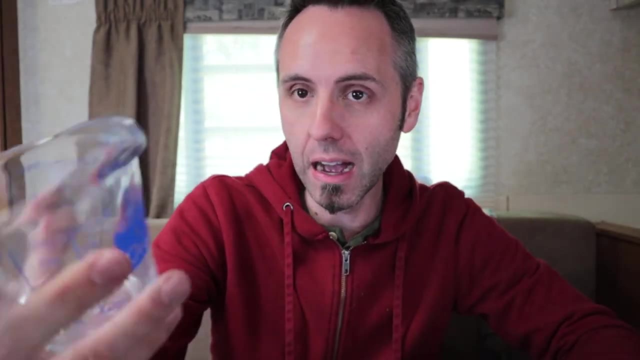 you guys are using and if that is causing it to lose its markings on there. We use finish mainly. We get it from Costco and we've been using it on this one. We haven't had any issues here. I'm kind of curious to see what's gonna happen here. 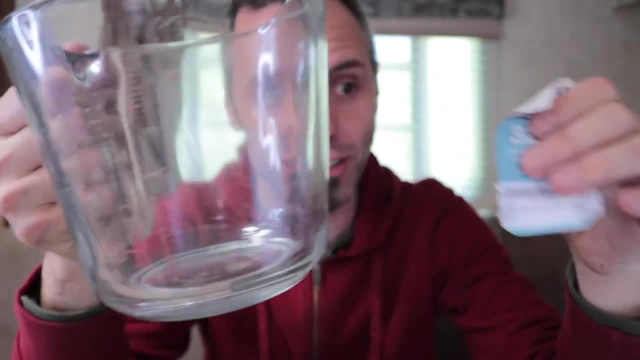 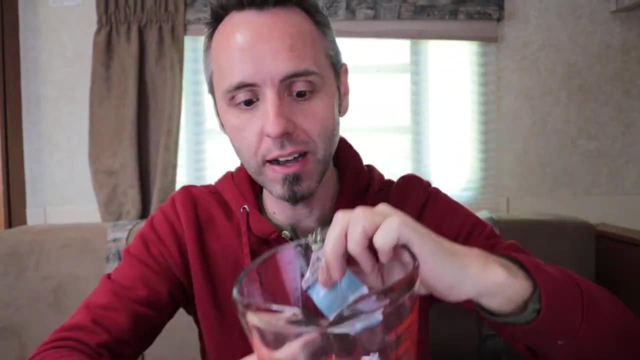 And we didn't have any. I mean, we did have issues with this one here, So that could be maybe finish wipes off the Pyrex one, but not the Anker Hawking one. I don't know. That's why I need to know from you guys down in the comments. 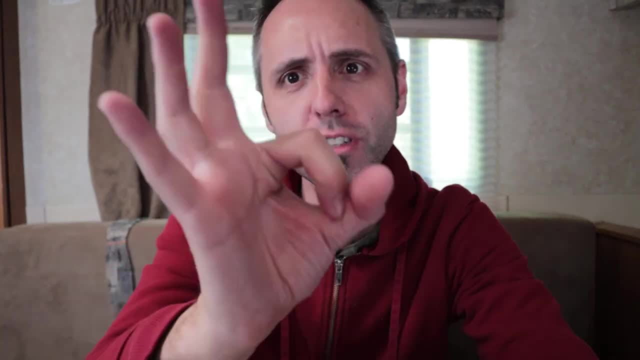 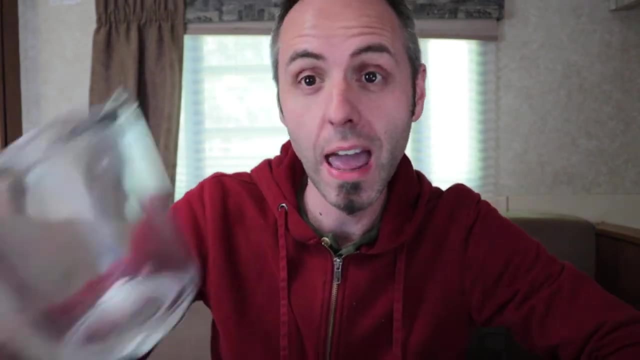 what kind of dishwasher detergent do you guys use? We use the little pods too, the little tabs. So let me know if it's a liquid or if it's a tab or if it's a powder. what kind of stuff you guys use? 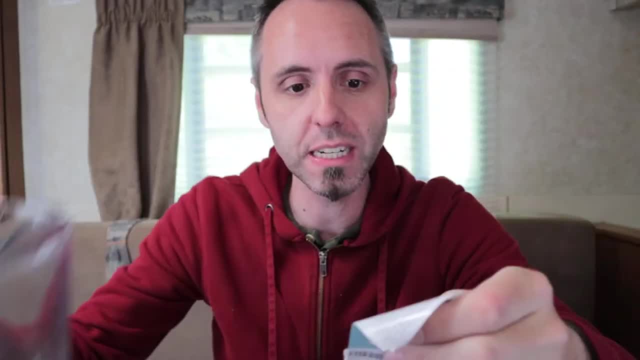 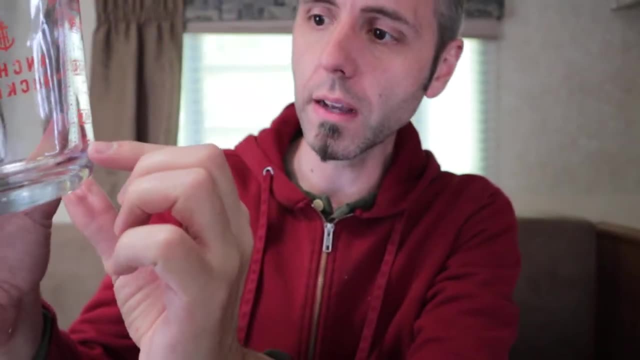 And let me know if y'all have a Pyrex or an Anker Hawking, if y'all are missing markings on there. That's all it says on the back of this thing here. Let's see, we're looking at this. It goes from one half cup all the way up to four cups. 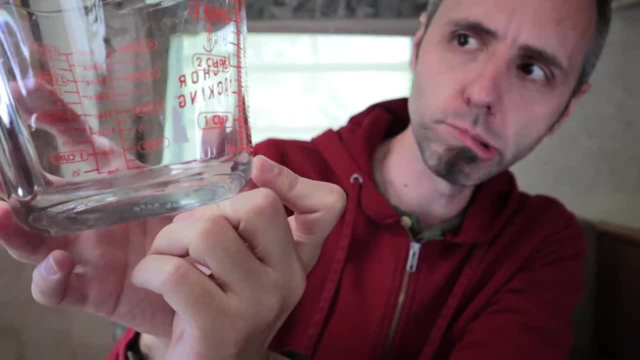 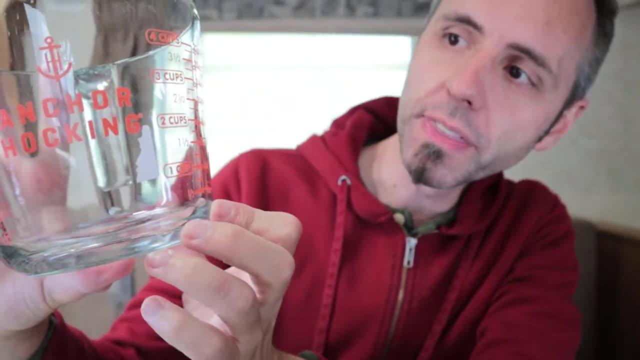 And then it goes from 100 liter of milliliters, 100 milliliters, to one liter right there, And then it has the same markings on the side here. but these go, they do cups, and then they do ounces, and then they do quartz as well. 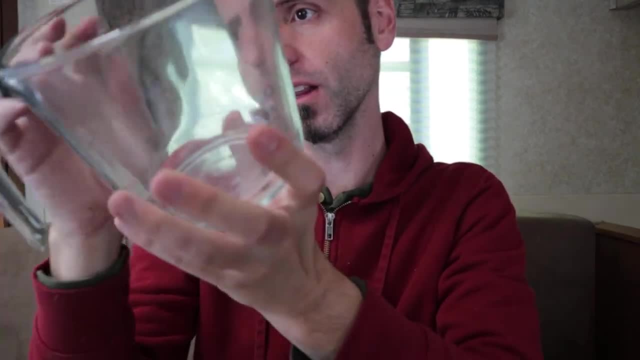 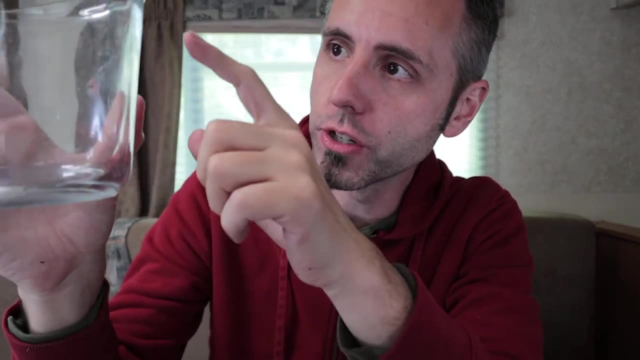 The Pyrex one. well, if I could read it, it doesn't look like there were any markings on this side. So this one only had the one to four cups And the 100 to one liter. It does. I can't. I don't see any markings on this side. 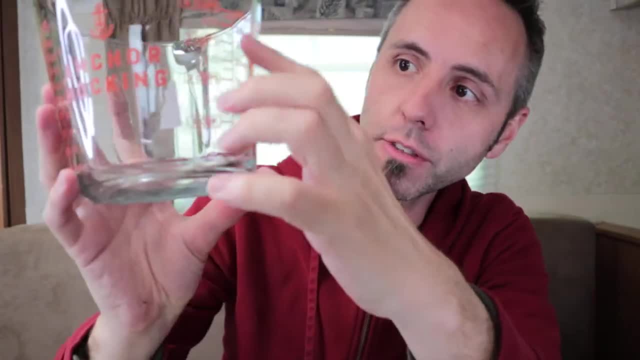 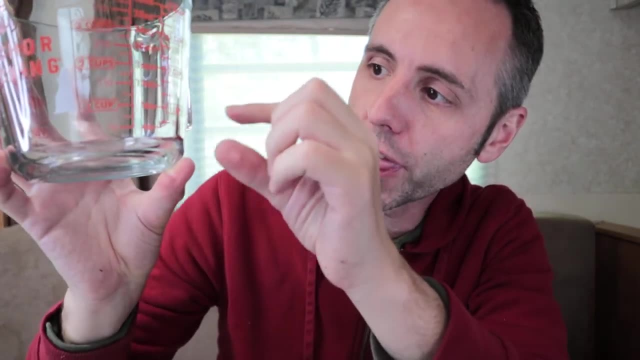 So this one has the plus in that it gives you your ounces, and these go by four ounces, So four, eight, 12,, 16,, so up to 32.. And then they give you the quartz, with a third of a quart. 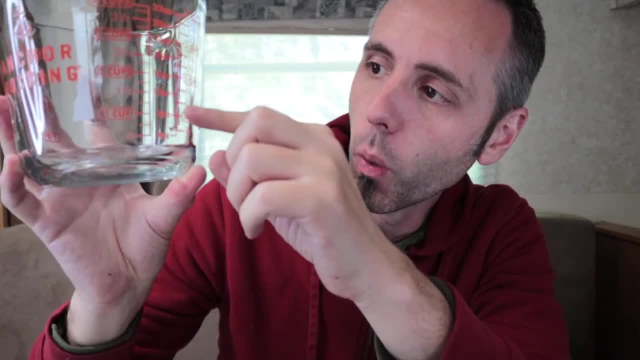 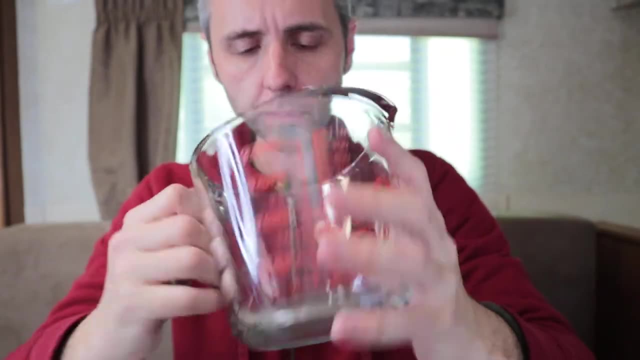 the lowest one being two thirds. but then it goes from one cup, one and one third, one and two thirds all the way up the scale there to the one quart. Let's see. As far as weight, these should be about the same. 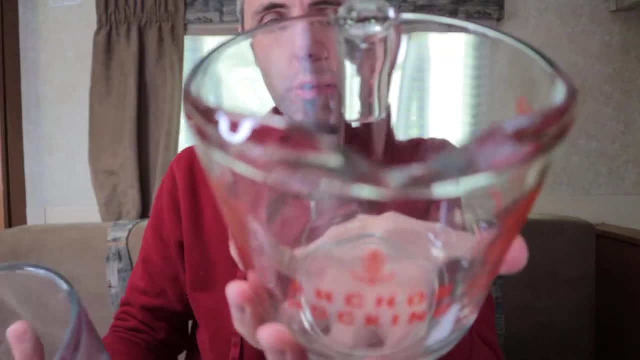 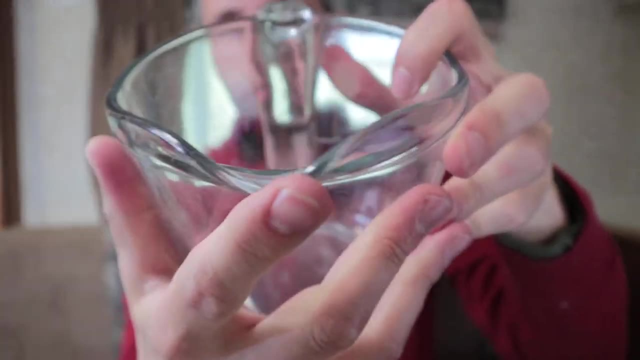 Yeah, I'd say that these are the same. They both have the spout on them too. Y'all can see the spout right there. It's got a nice little lip to be able to let your liquids flow out of there. Same thing with this one here. 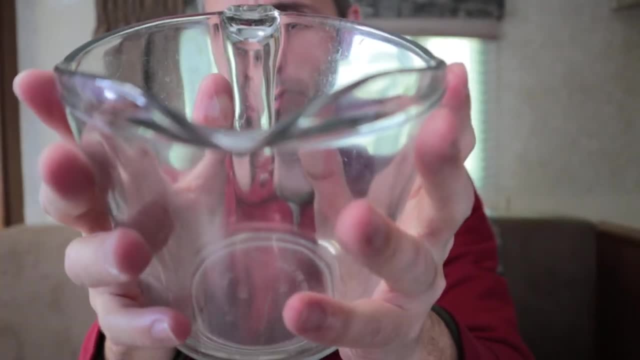 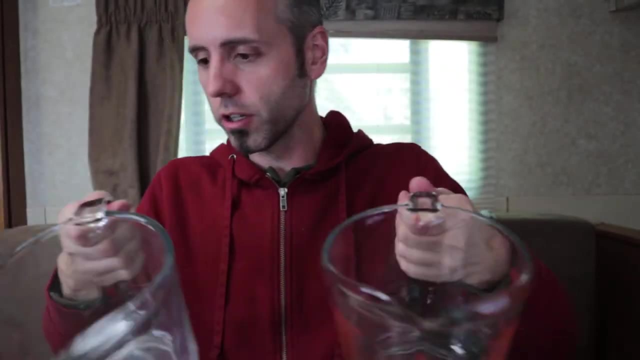 the old Pyrex one that we had. This one looks a little warped, Is that a little that could? huh, That's interesting, Maybe not. Maybe that's just from the stem on the back here, the handle, As far as the handles are concerned, looking at those. 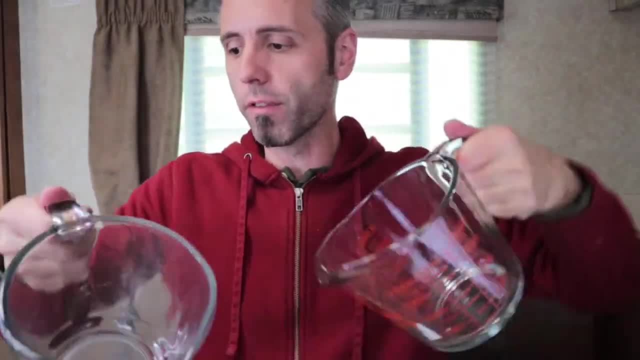 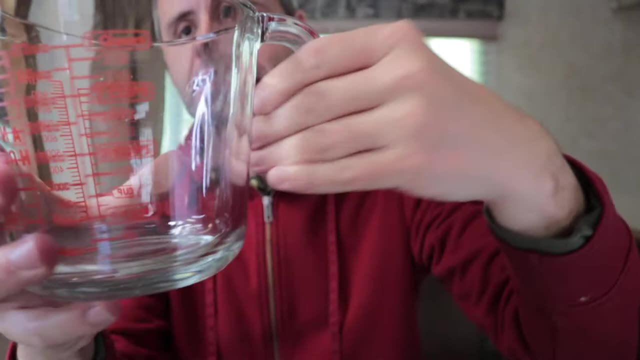 they both have a nice little divot right here so that you can put your thumb, so that whenever you're pouring, both of them are just flat on the back. So they're not ergonomically designed for your fingers, but it is this nice smooth glass texture. 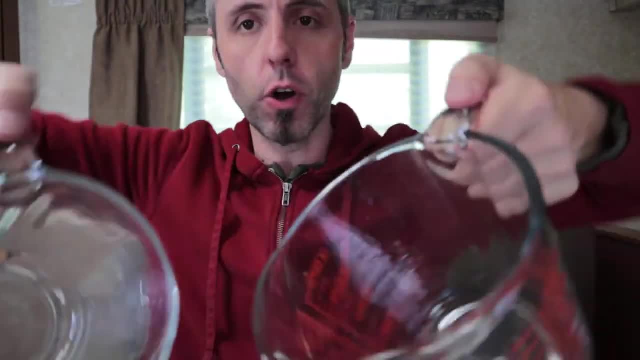 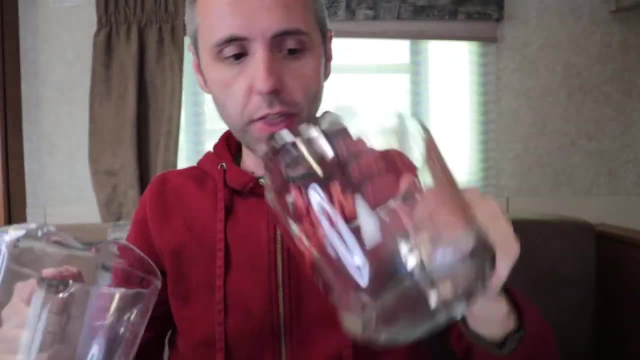 So that's not too much of an issue, but it does have a little divot on the top here as well. So a place to where you can put your thumb and have a little bit more control over your pour. The bottoms of them. they look to be about the same. 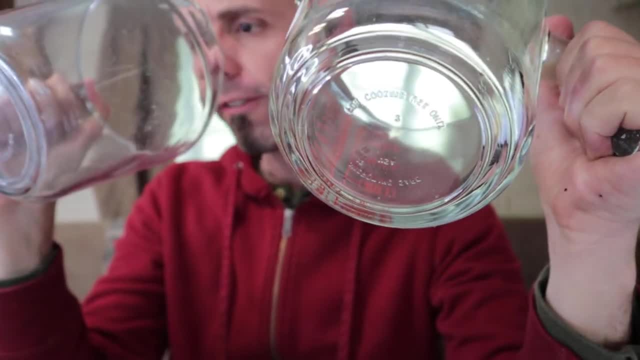 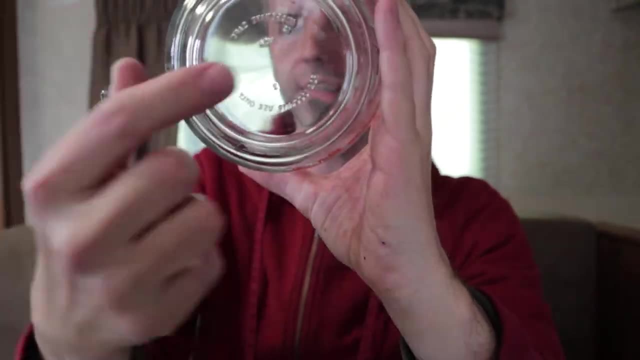 This one says Microwave Safe- USA- 24 for cooking use only, And this one says Microwave Safe- USA for cooking use only, And this one has a number 19.. I don't know what those little numbers mean. This one has a 20..